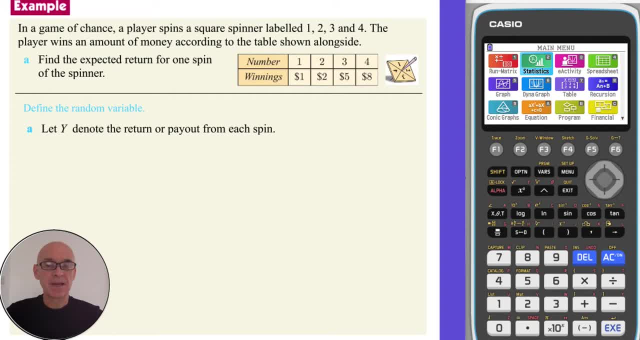 We'll let y equal the return or the payout from each spin. As it's a square spinner, the probability of each outcome is a quarter And the probability distribution of the payout, y, is shown in the table here. To find the expected return, we use our formula for the expected value. 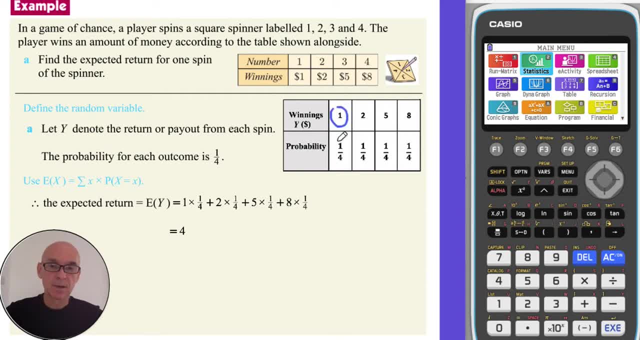 And again, that's found by multiplying each of the winnings by their respective probabilities. So the first case, one multiplied by a quarter, then two multiplied by a quarter, and adding up each of those calculations, So you can see, the expected return is four and that's four dollars. 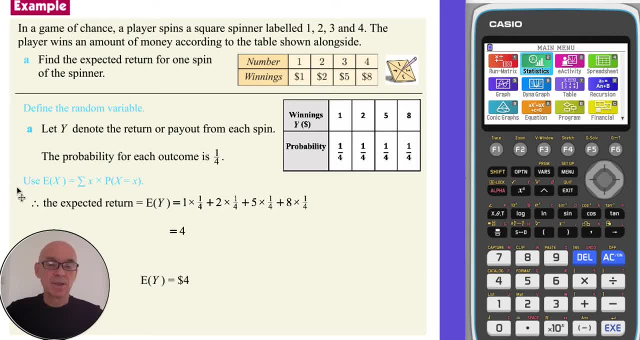 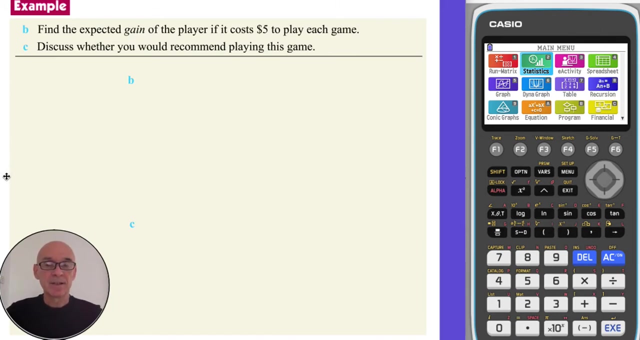 Again, if you wish, you can type the probability distribution into the lists of your calculator and the calculator will calculate the expected value for you, as shown to the right here. Now to find the expected return, To find the expected gain of a player: if it costs five dollars to play each game, we 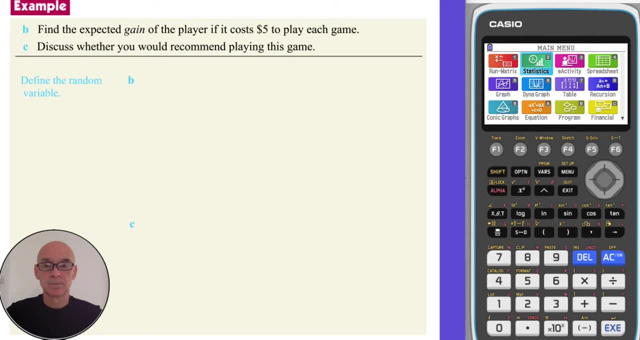 define a random variable. So we'll let x denote the gain of the player from each game, And since it costs five dollars to play the game, then the expected gain is found by subtracting the cost from the payout. Four subtract five is minus one dollar. 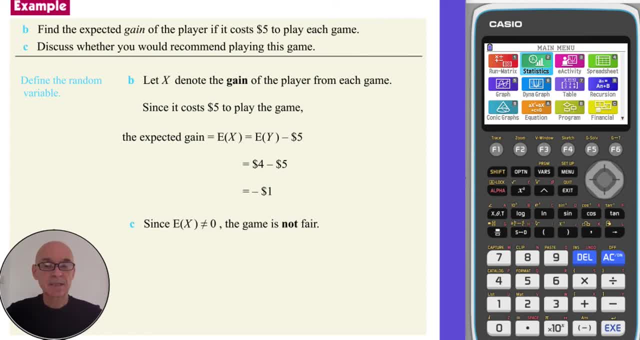 So that's the expected return. So since the expected gain is not equal to zero, the gain is not a fair gain. So since the expected gain is minus one dollar, that means we would expect the player to lose a dollar on average with each spin. 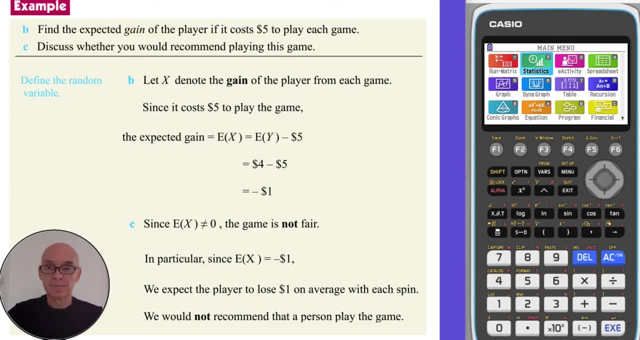 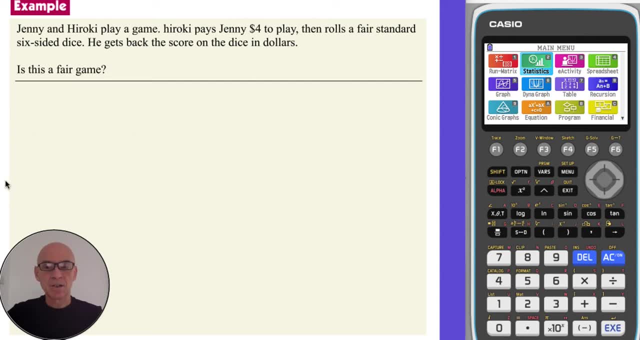 So we would not recommend a person play the game. In this question we're asked to decide whether the game is fair. So, again, if we start by defining a random variable, we'll let x be the score on the dice And to calculate the expected payment, again we use our formula.